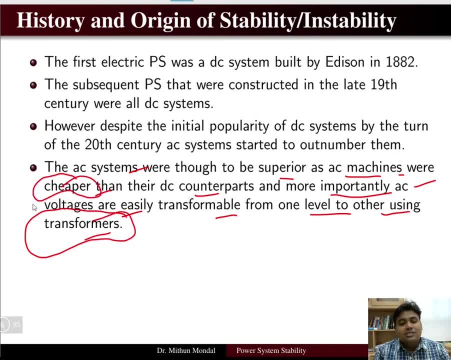 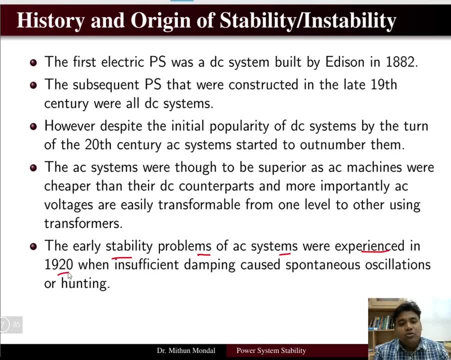 voltage and also the AC machines are cheaper as compared to the DC machine. The early stability problem of AC system were experienced in 1920 when insufficient damping cause in spontaneous oscillations or hunting. So the stability problem were first observed in 1920 when there was 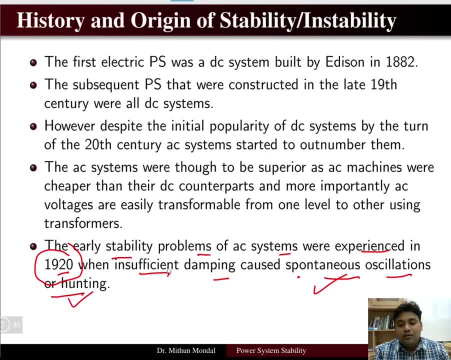 spontaneous oscillations or hunting in the machine. These problems were solved using generator, damper winding or use of turbine type prime mover. So, although the initial problem early occurred as 1920 with the AC system due to which the hunting has occurred, this hunting was 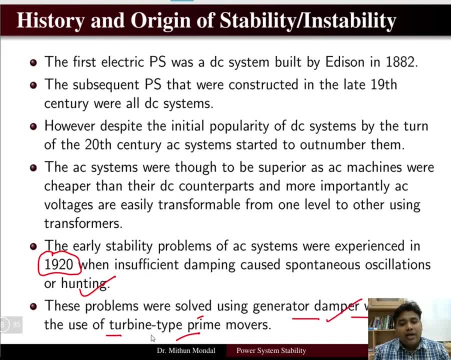 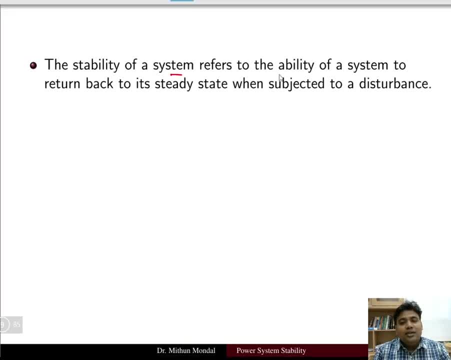 solved using damper winding and the use of turbine type prime mover. The stability of a system then referred to the ability of a system to return back to its steady state. So the stability of a system then referred to the ability of a system to return back to its steady state when subjected to a disturbance. 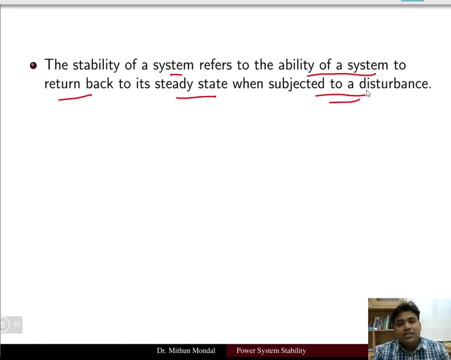 So, basically, any power system will be subjected to any disturbance. Then how do we define the stability? It is the return of the system to the steady state. Conversely, instability means a condition denoting loss of synchronism or falling out of state. So stability when it is returned. 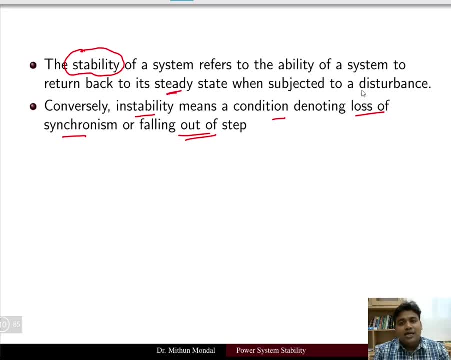 back to the steady state after the disturbance has been resolved, whereas instability is falling out of the original condition and decreasing of the motion. withanı go behind such a shock absorber or shock fan falling out of step or loss of synchronism. Power is generated by synchronous generator. 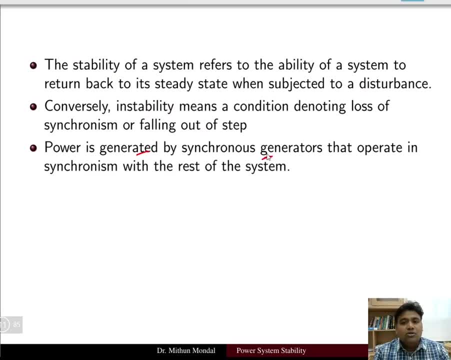 We know that the power is basically generated by three-phase synchronous generator or the alternator that operate in synchronism with the rest of the system. So we know that in power system many number of synchronous generators are connected in parallel and they will be in synchronism with the rest part of the system. So a generator is synchronized with a bus. 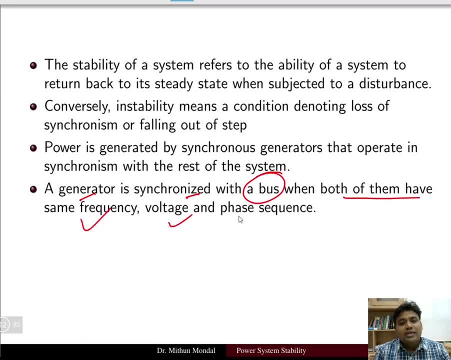 with when both of them have same frequency, voltage and phase sequence. So generally we make this condition: where we generators should have same frequency, it should have same terminal voltage and its phase sequence should be same. then only we can say that the generator is synchronized with a bus. We can thus define the power system. 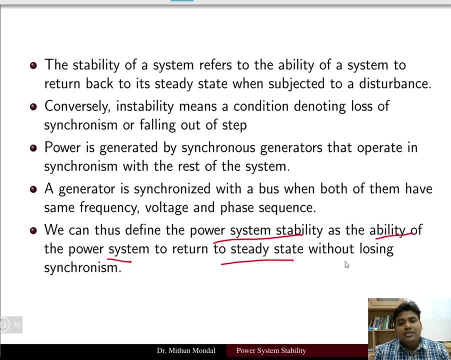 sequence as follows. We can thus define the power system sequence as follows: We can thus define the power system sequence as follows: We can thus define the power system sequence as the ability of a power system to return to steady state without loss of synchronism. 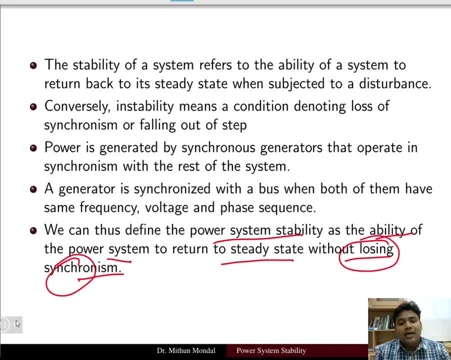 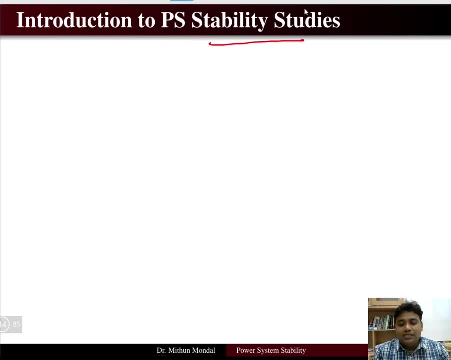 So this losing of synchronism basically means that any generator is losing its frequency, voltage or phase sequence and then it is coming out of the step. So introduction to power system stability studies. What is stability? we have defined It is refers to stable operation of the synchronous machine connected. 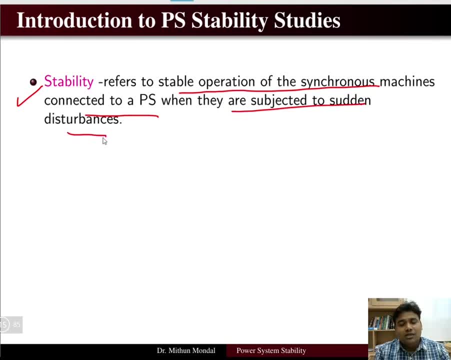 to a power system when they are subjected to sudden disturbance. So any synchronous machine, when subjected to disturbance, if it is returning to the stable state, then it is known as stability. Stability is the ability of a power system to return to stable operation when subjected to a 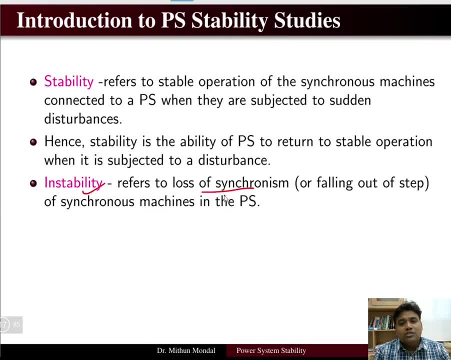 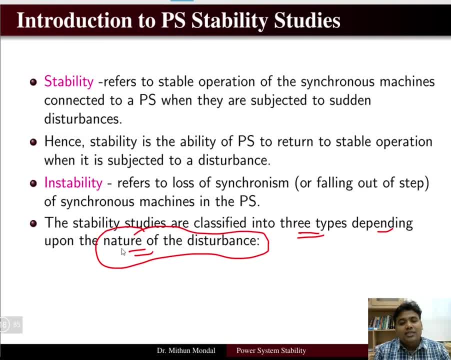 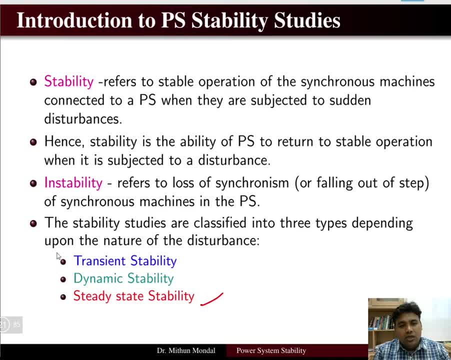 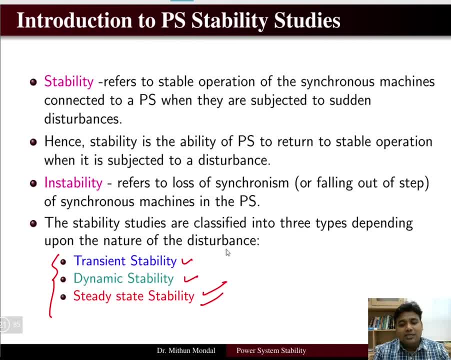 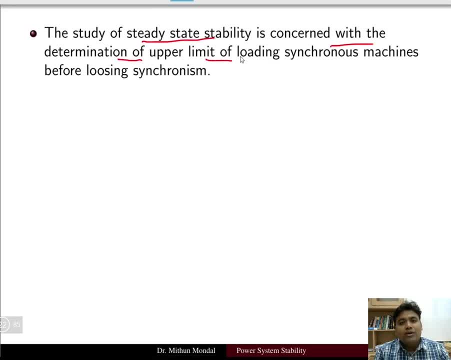 depending upon the nature of the disturbance, The stability studies are classified into three types. depending upon the nature of the disturbance, The stability studies are classified into three types. occur due to the variation in the load, changes in the speed of the prime mover, or fault in the 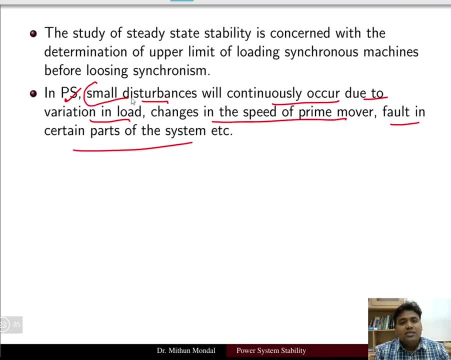 certain part of the system. So we can't omit the disturbance. So disturbance will always be there in the power system and that is because of the variation in the load change, in the speed of the prime mover or fault in certain part of the system. These small disturbances may excite the system. 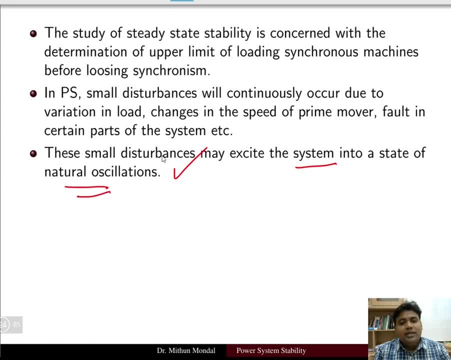 into a state of natural oscillation. So whenever there is a disturbance it will try to produce a oscillation in the circuit which is the natural oscillation. In dynamically stable system the amplitude of oscillation will be small and they die out quickly. So if the oscillation which is 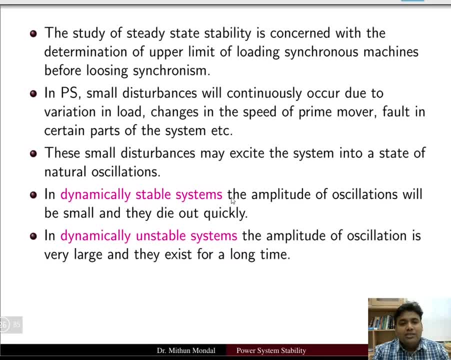 produced due to disturbance die out, then it is known as dynamically stable system. However, in dynamically unstable system, the amplitude of oscillation is very large and they exist for a long time. So here, when it is dying out the natural oscillation, it is exist for a long time. 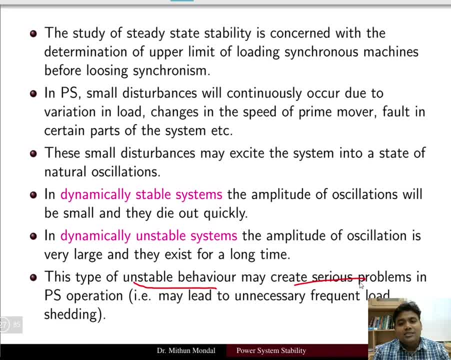 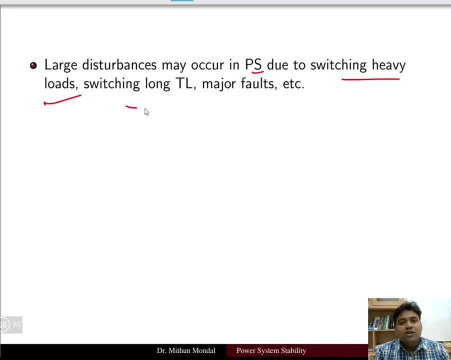 These type of unstable behavior may create serious problem in power system operation and they can be unnecessary, frequent load shedding. So whenever you have either dynamic, stable or unstable systems, then there will be serious load shedding and of the problem, Large disturbances may occur in power system due to switching heavy loads, switching long transmission line and major fault. So we 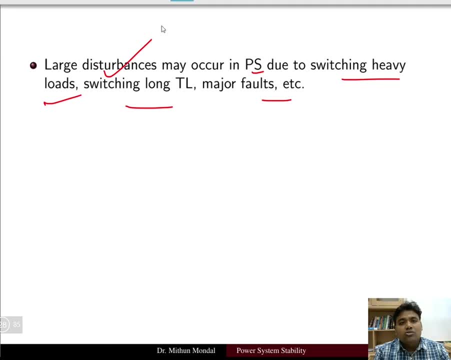 have seen the small disturbances and large disturbances can also occur in the power system. Rarely when there is a fault in the power system or when we switch on the heavy load. The sudden large disturbances are characterized by large changes in the speed of the rotor of the synchronous motor. 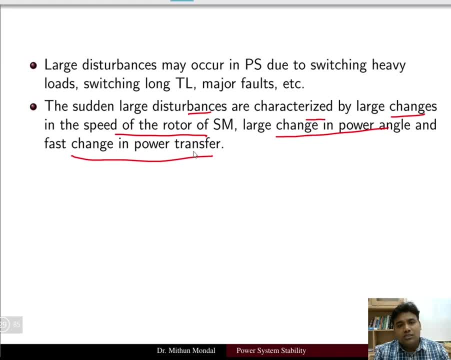 large change in the power angle and fast change in the power transfer. So wherever there is a large disturbance in the power system, you will observe that the speed of the rotor of a synchronous motor has changed, or there is a large change in the power angle- that is delta- and if there is a change in the 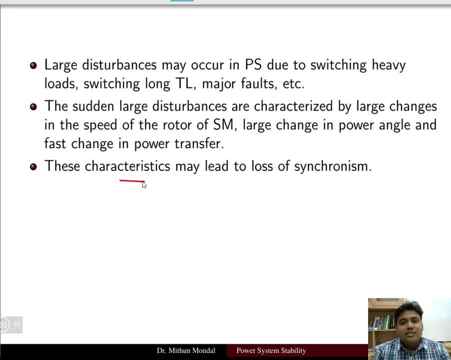 power angle, then there is a fast change in the power transfer. These characteristic may lead to loss of synchronism. So again there can be loss of synchronism because of this large disturbance. This type of instability is called transient instability. So whenever there is a large 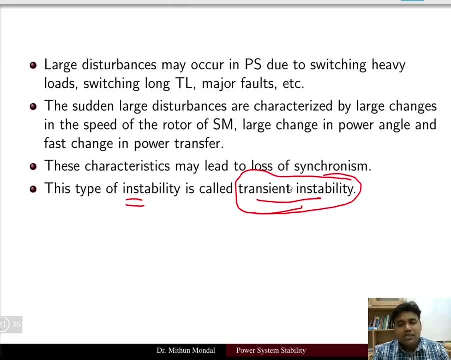 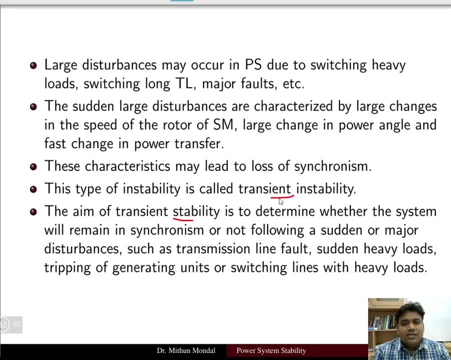 disturbance, there will be loss of synchronism and this instability is called as transient instability. The aim of transient stability. So this is transient instability, and the aim of transient stability is called as transient instability, And the aim of transient stability is to determine whether the system will remain in synchronism or not. 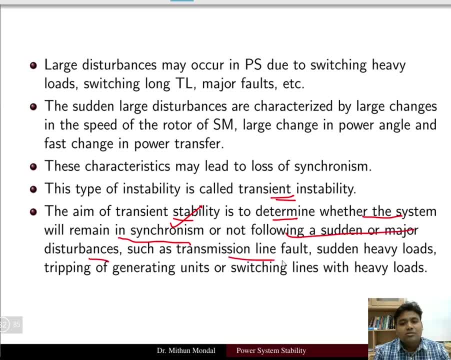 following a sudden or major disturbance, such as transmission line fault, sudden heavy load, creeping of generating unit or switching lines with heavy load. So these are basically the large disturbance that we are talking about. and then what is the aim of the transient stability is to 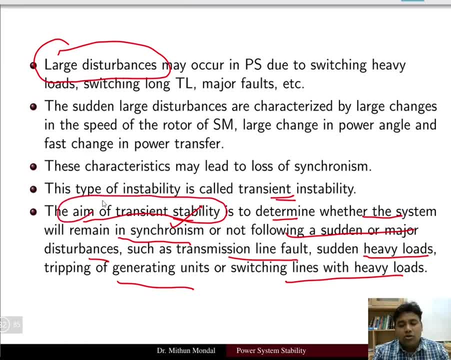 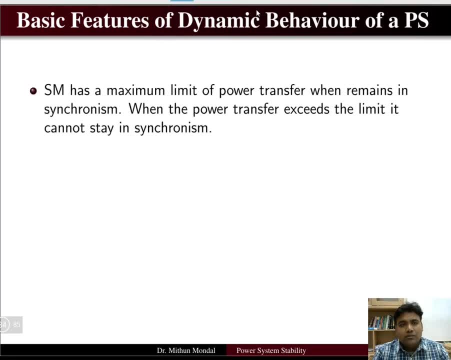 determine whether the system will remain in synchronism or not when a large disturbance has occurred. So there are certain features of dynamic behavior of a power system. So the first behavior is synchronous machine has a maximum limit of power transfer when remains in synchronism. So whenever the synchronous machine 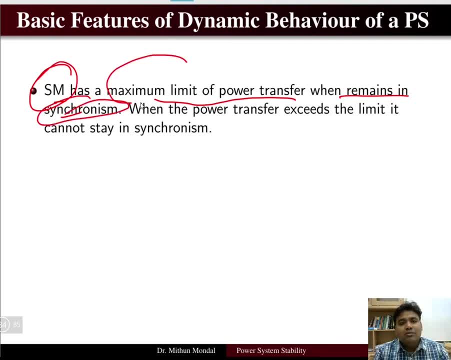 will be in synchronism state. then only the maximum limit of power transfer will occur. When the power transfer exceeds the limit, it cannot stay in synchronism. So we can see the graph of the power. So the graph of the power is like this. So we have with respect to delta. 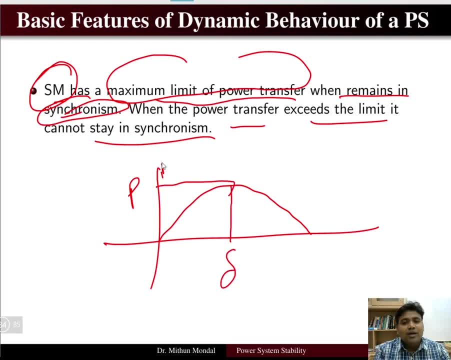 Then the power will be maximum. So here we have the maximum power. This we will look ahead. So power will be maximum only when it remains in synchronism. Power can be more than the synchronism also, and it can lose the synchronism. That is what. So this is known as power delta curve, which we will look 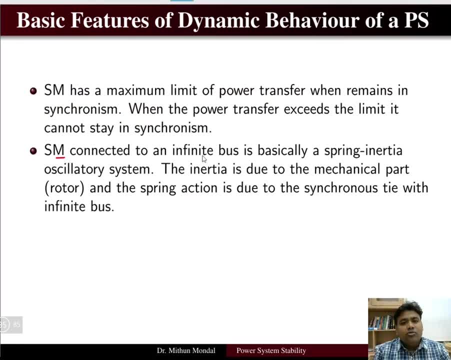 ahead. Synchronous machine connected to an infinite bus is basically a spring, inertia oscillatory system. So we know that in the mechanical system we have a spring which is connected with a infinite bus. So spring and inertia, So it is basically same thing. If you have a synchronous machine then you are connected with a bus. So we study the 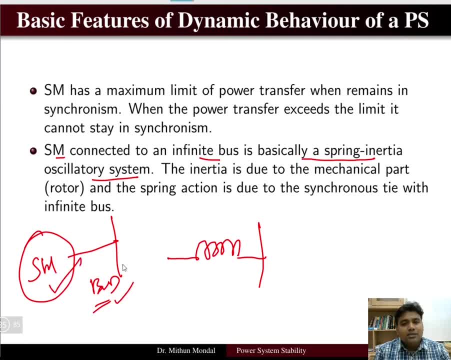 stability studies in terms of synchronous machine connected with a bus. So here we say that synchronous machine connected with an infinite bus. Why infinite bus? Because here the voltage will be constant and frequency will be constant for the bus, So it is known as infinite bus. It is basically a spring inertia oscillatory system. The inertia is due to the 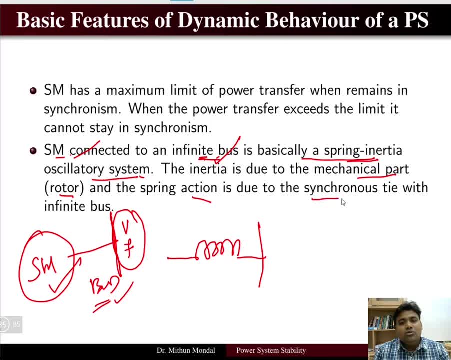 mechanical part, the rotor and the spring action is due to the synchronous tie with the infinite bus. So you have a synchronous tie of the synchronous machine with respect to the bus. Bus is infinite, So the voltage and frequency remain constant and the inertia is due to the 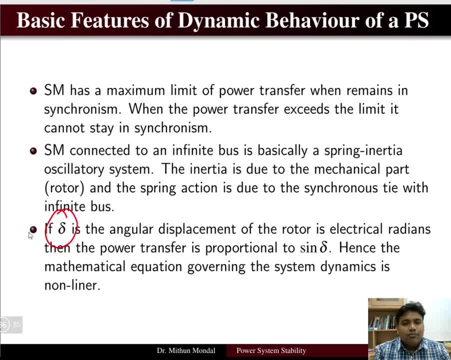 mechanical part, that is the rotor. If delta, that is the power angle, is the angular displacement of the rotor in electrical radian- sorry, here delta is representing the angular displacement of the rotor in electrical radian- then the power transfer is proportional to sine delta. So power transfer will be proportional to: 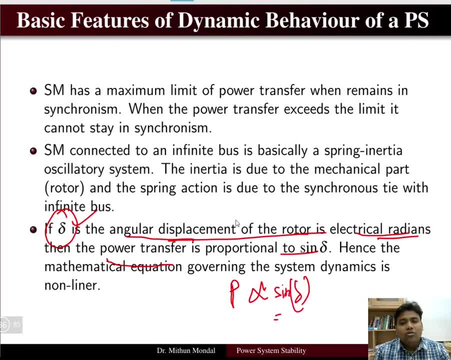 sine delta, and delta is basically the angular displacement of the rotor in electrical radian. Hence the mathematical equation governing the system dynamic is non-linear. So here we see that the power is a function of sine of delta. So the dynamics that will refer the mathematical 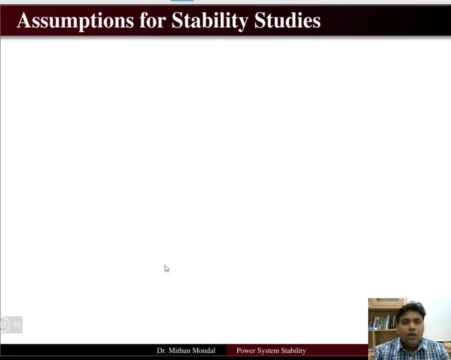 equation will be non-linear. There are certain assumptions that we will do to study the stability. First assumption is that the DC offset, current and harmonic components are neglected. We will not include the DC offset, current or harmonic component. The current and voltage are assumed to have the fundamental component alone. So generally we know that. 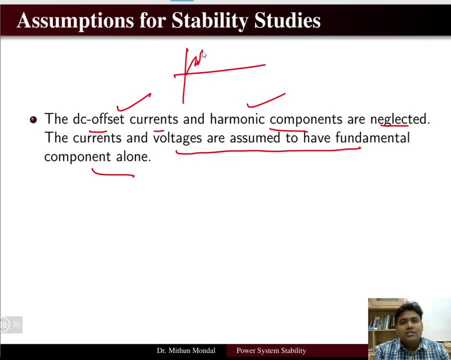 if you have a current, then always there will be some harmonics present. So the harmonics and DC offset current will neglect and only the fundamental component will take into consideration. The symmetrical components, which we have already studied, will be used for representation of 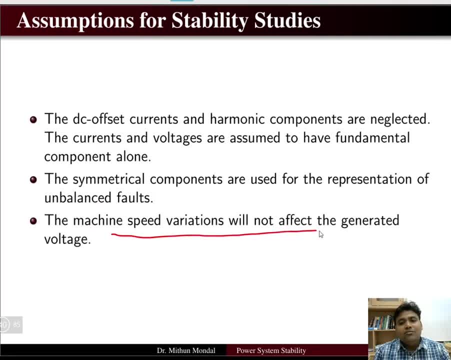 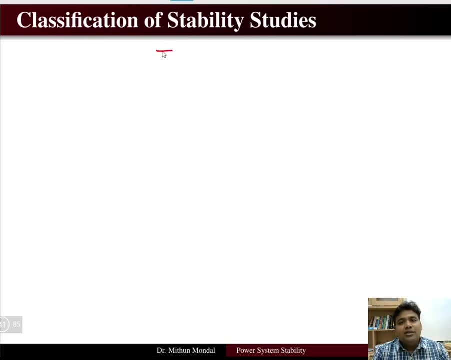 unbalanced faults and the machine speed variation will not be affected by the generated voltage. So whatever the speed machine varies, it will not affect to the generated voltage. So these are basically the assumptions that we will take in stability studies. Let us classify the stability. 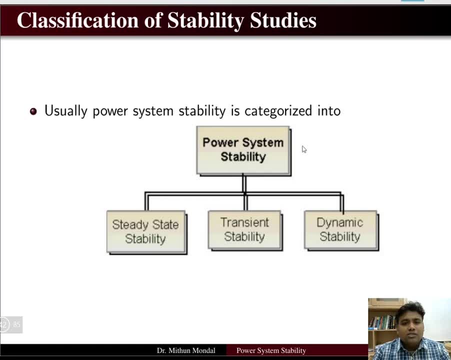 studies, which we will see in the next issue. So let us see the stability studies that we will see. we have already studied. So power system stability will be classified as steady state stability, transient stability and dynamic stability. We have looked a little bit back. 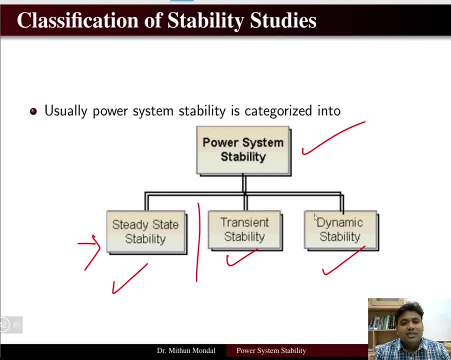 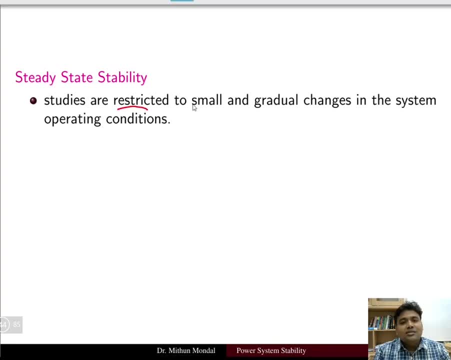 and we have seen what is the difference between a steady state stability, transient stability and dynamic stability. However, let us look more into it. So steady state stability are the studies which are restricted to small and gradual change in the system operating condition. So, whenever 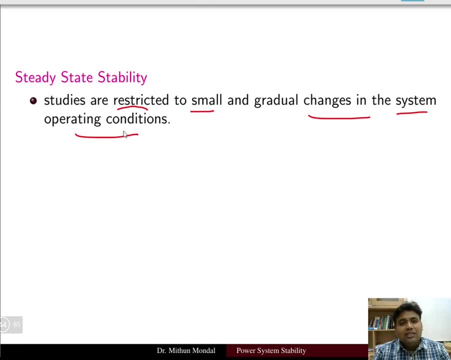 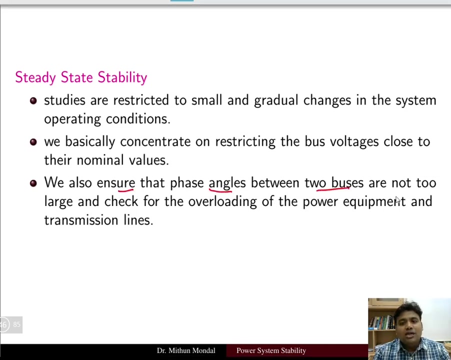 your system is having a gradual change, then that type of studies are known as steady state stability. We basically concentrate on restricting the bus voltage close to their nominal values. We also ensure that the phase angle between the two buses are not too large and check for the 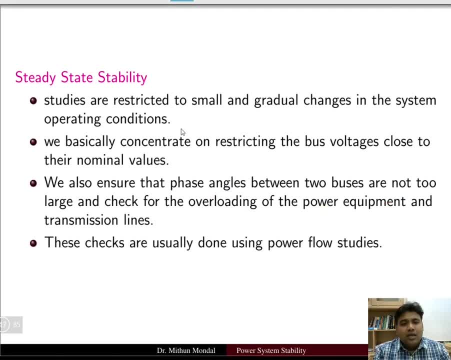 overloading of the power equipment and transmission lines. In these we check, usually done using power flow studies. So power flow studies we have done using Gauss-Seidel or Newton-Raphson method So that methods will be used to check whether the 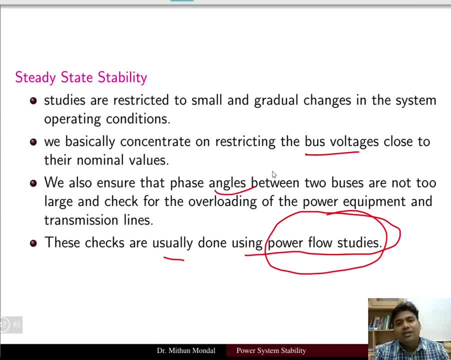 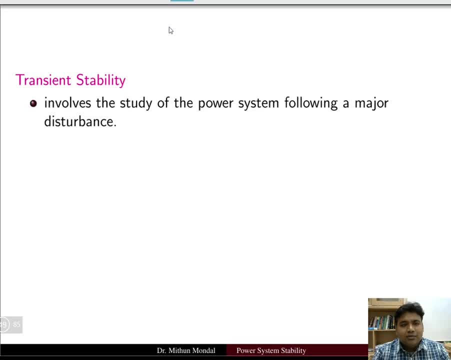 voltage, that is, the bus voltage or the phase angle, are not varying a lot, and there is a gradual change in the operating conditions. Now let us see the transient stability. So transient stability basically involves the study of our system following a major disturbance. So whereas in 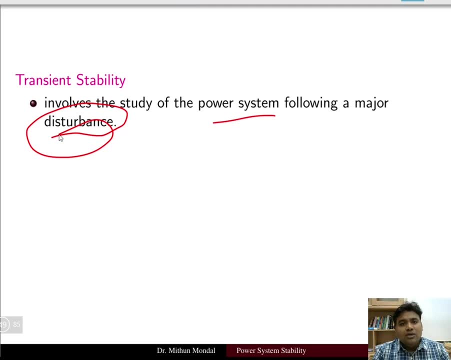 steady state, stability. the disturbance is minute. here you have a major disturbance. So, following a large disturbance, you have a major disturbance. So following a large disturbance, you have a major disturbance. So, following a large disturbance, the synchronous alternator, the machine power. 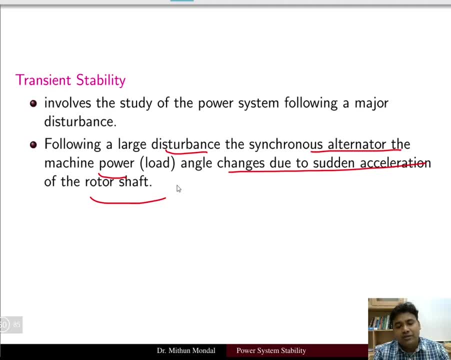 angle changes due to sudden acceleration of the rotor shaft. So we have seen that when there is a large disturbance in the power system due to the fault or sudden switching of the heavy load, then there will be heavy change in the power and also there will be in machine power. angle will be. 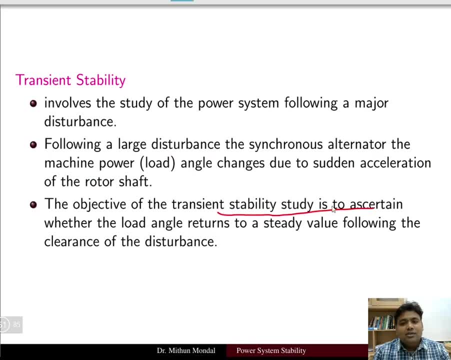 changing. The objective of transient stability study is to ascertain whether the load angle return to the steady state value following the clearance of the disturbance. So we have seen the load angle delta here. So the load angle delta here, do it return to the steady state? 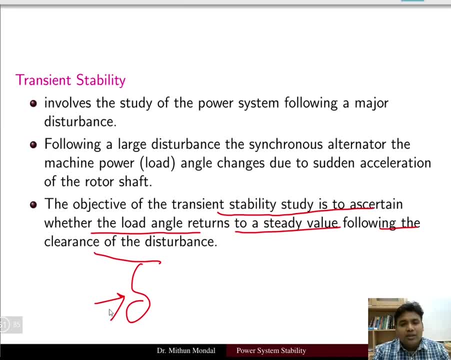 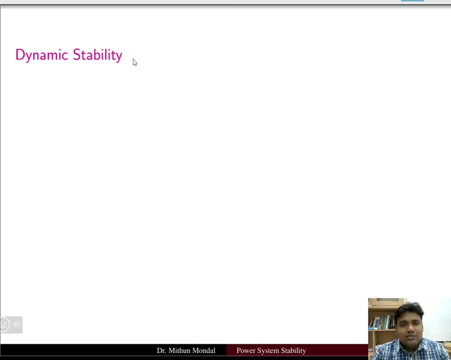 stability or the steady state value when the disturbance has been removed. So that is the objective of transient stability. There is other stability that we have seen. that is the dynamic stability, So the ability of a power system to maintain stability under the continuously small 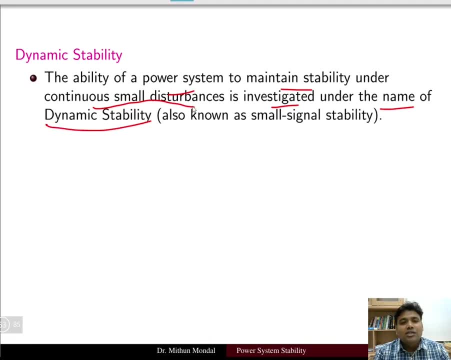 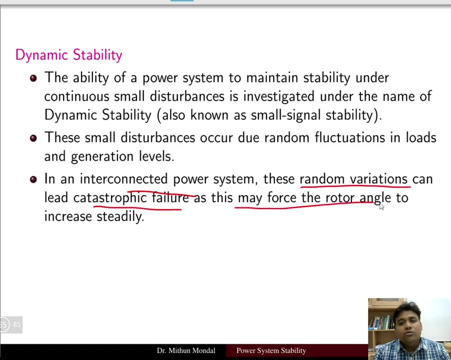 disturbance is investigated under the name of dynamic stability, also known as small signal stability. These small disturbances are called dynamic stability, So the dynamic stability is called dynamic stability. due to random fluctuations in loads and generation levels In an interconnected power system, these random variation can lead to catastrophic failure, as this may force. 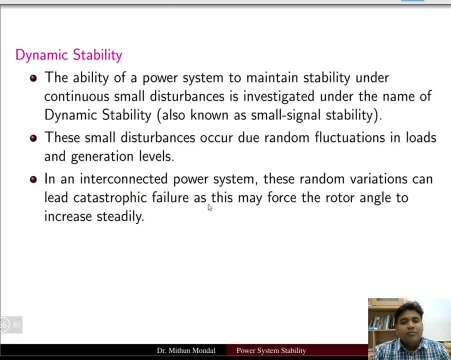 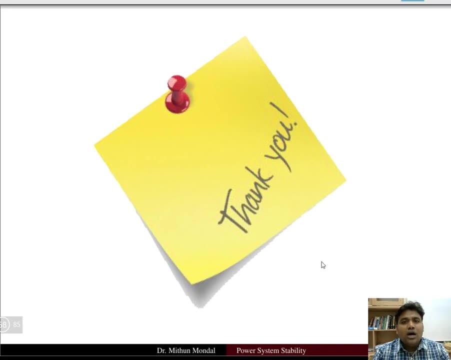 the rotor angle to increase steadily. Basically we will be focusing our study on the transient stability studies for the power system. So we have seen the different stability studies in power system and we will focus our study on transient stability and we will see why the machine lose its synchronism and what happened and what are the different terms. 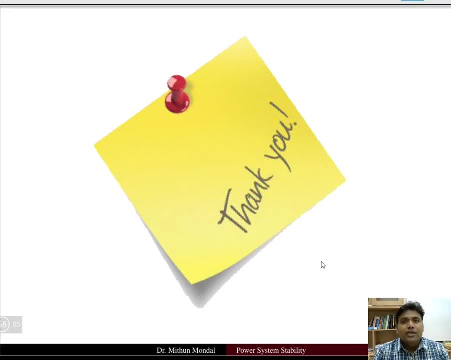 and conditions for the power system stability. Thank you. 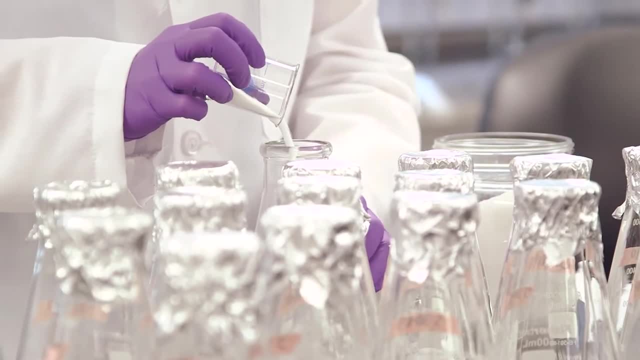 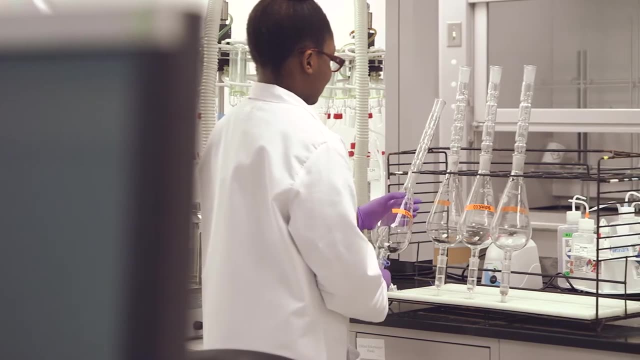 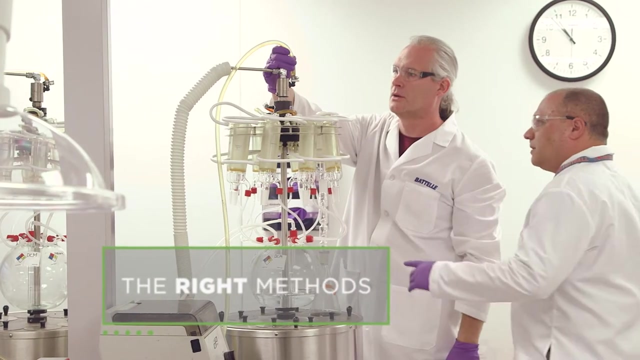 When it comes to analytical chemistry, especially when you need more than standard testing services, you can always count on Battelle. In fact, Battelle goes beyond standardized analytical testing to help you better understand your data and select the right methods to solve your specific problems, Backed by a deep understanding of environmental science. 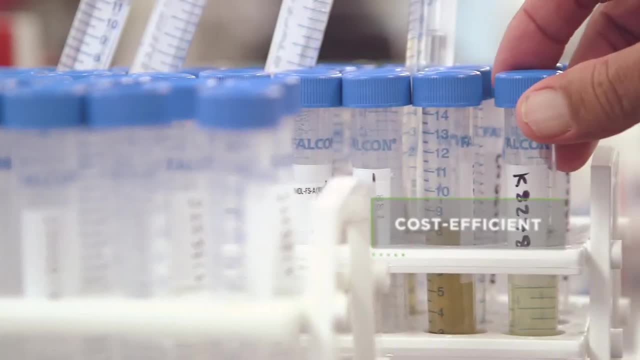 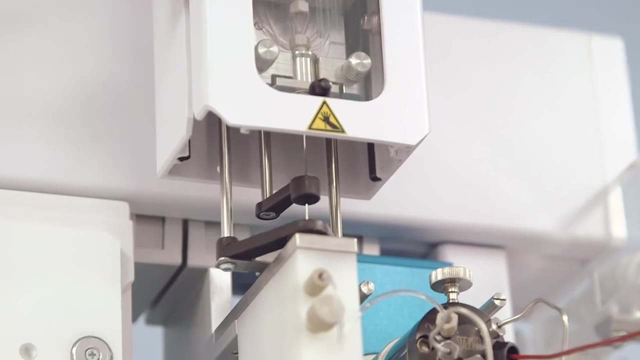 we can help you find the most effective and cost-efficient path to the solutions you need, And if the right method doesn't exist, we'll help you develop it. That's because Battelle brings together world-class analytical laboratory services with expertise in environmental science. 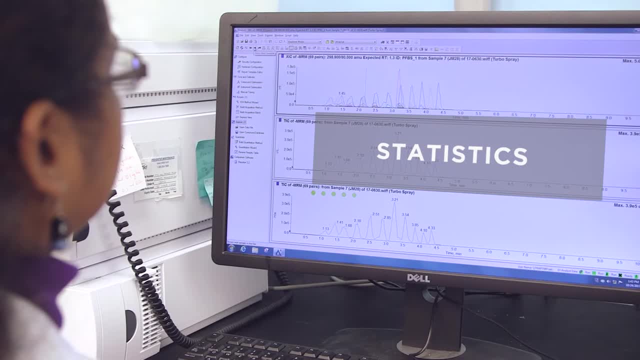 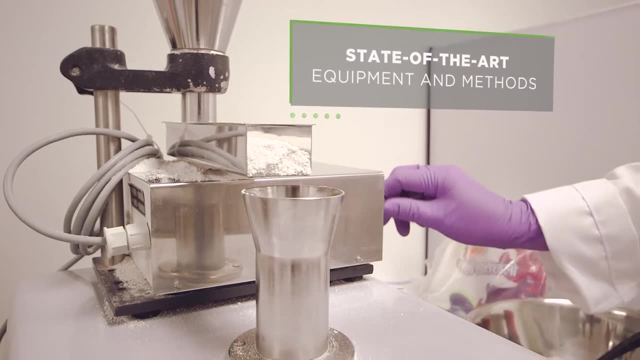 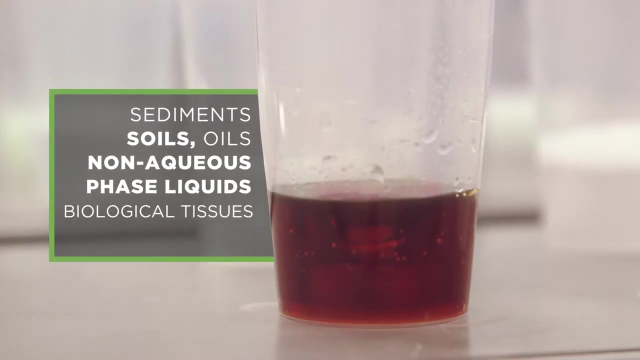 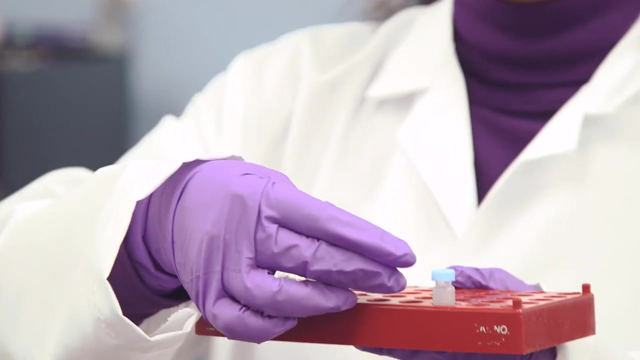 toxicology data, analytics and statistics. Our broad range of services include: analytical lab services, state-of-the-art equipment and methods to accurately measure contaminants in sediments, soils, oils, non-aqueous phase liquids, biological tissues, water, air and food. Chemistry consulting, Expert guidance for method selection or data. 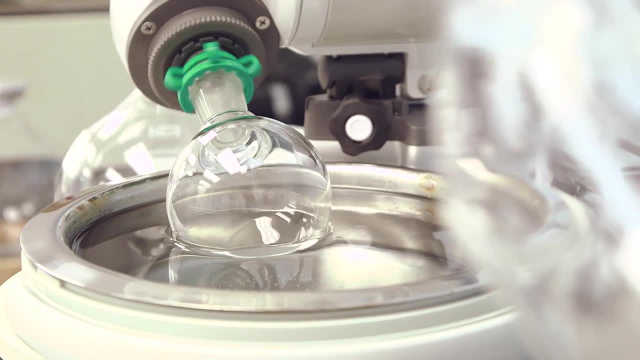 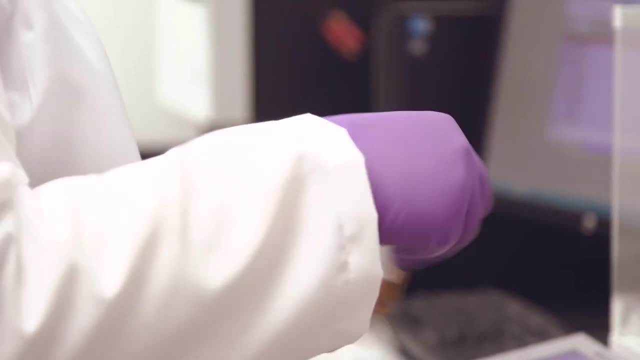 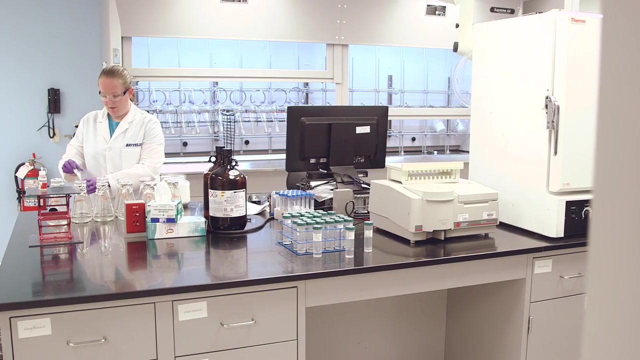 interpretation, Working with you to design a study plan that addresses your specific questions and challenges. And method development and optimization. Rigorous methods for complex analytical needs and non-standard problems that go beyond standard EPA methods. Don't just settle for data When you need real answers to your analytical chemistry challenges – answers. 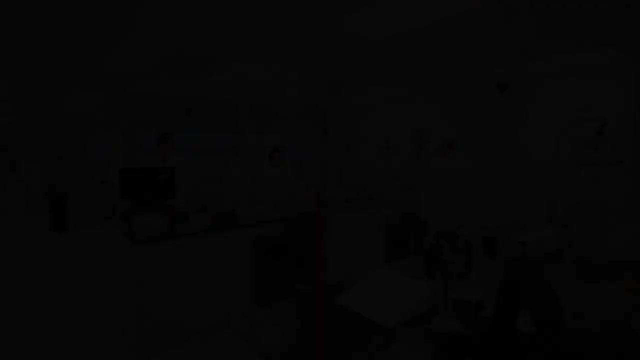 tailored for your specific needs. We can provide you with an overview of the solutions scientific need, because at Battelle it can be done.